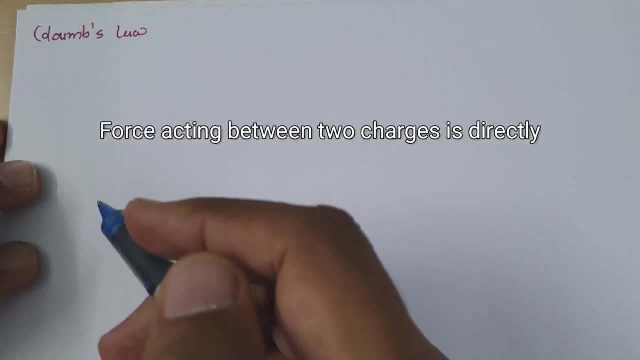 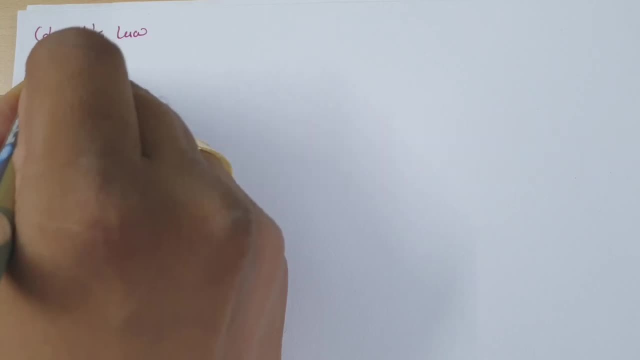 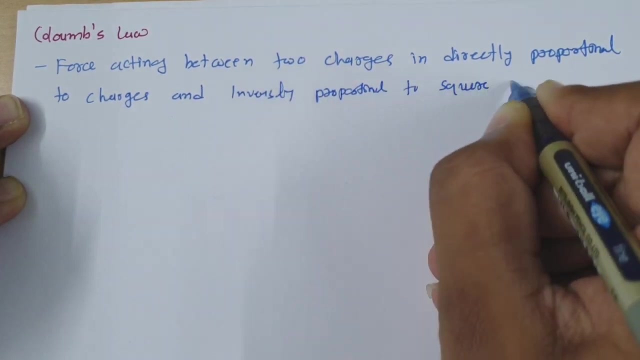 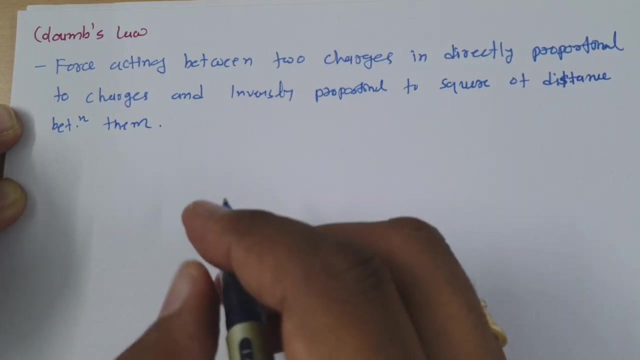 between two charges that is directly proportional to their charges and inversely proportional to square of the distance between them. So let me write it So: force acting in between two charges that is directly proportional to those two charges and inversely proportional to square of distance between them. So, for example, if I consider: 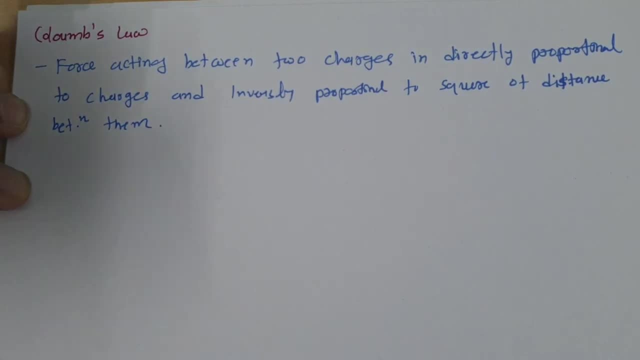 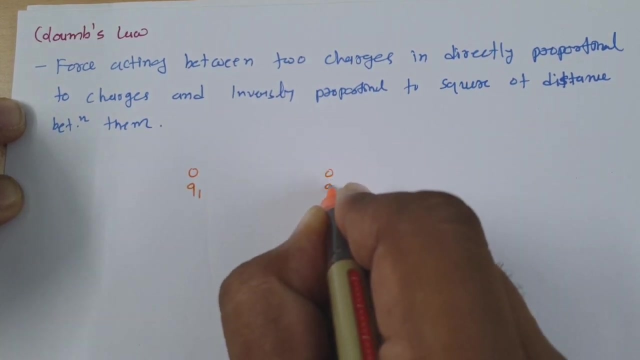 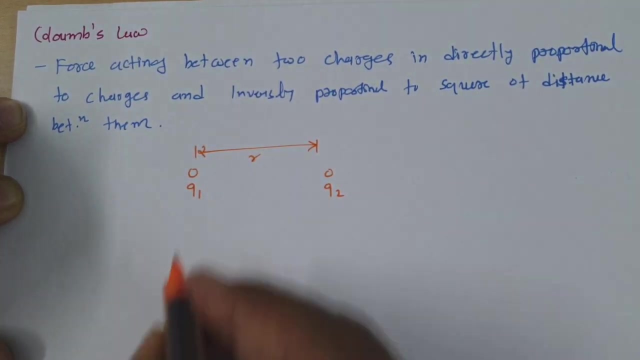 two charge particles. let us say one charge is Q1 and second charge is Q2.. And if distance between these two charges, that is if I say if it is R, then force acting between two charges will be 4.. force acting in between two charge particle. force acting in between these two charge particle. 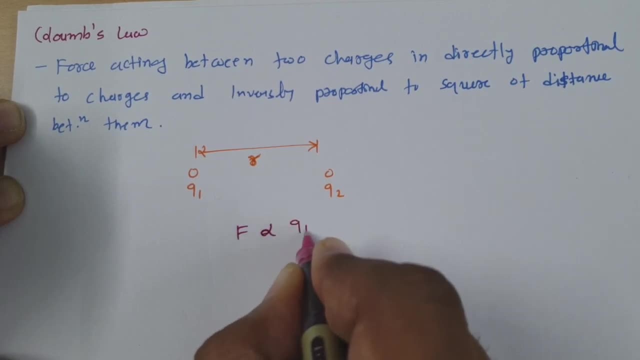 that force is directly proportional to this two charge, q1 and q2, and inversely proportional to square of distance between them. and this proportionality constant, this proportionality constant that is 1 by 4, pi, epsilon 0, and this is q1, q2 divided by r square. so this is coulomb's. 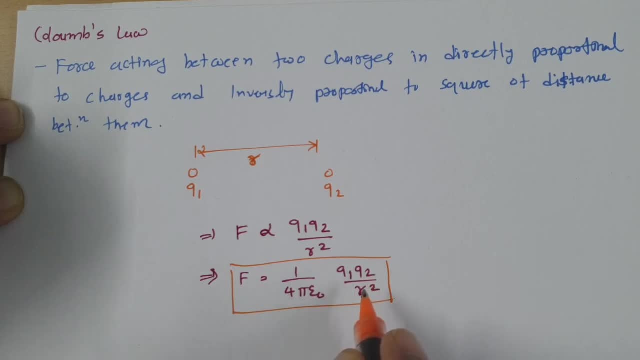 law, so force acting in between two charge particle that is directly proportional to those two charges and inversely proportional to square of distance between them. now i'll explain you two cases where what will happen if polarity of two charges are same. and second case will be: what will 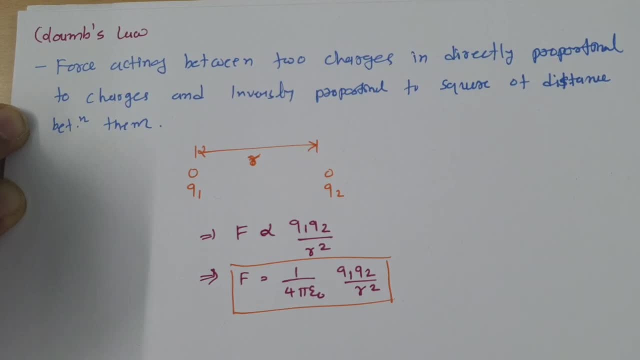 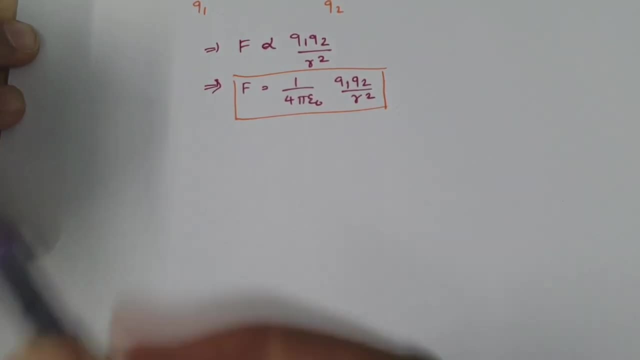 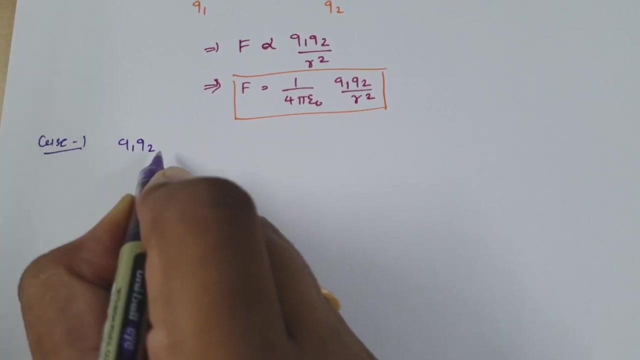 happen as if polarity of these two charges are opposite. so let us consider first case. so in first case, case number one, i'll consider both charges are having same polarity. so if both charges are having same polarity, like if both are positive, then they will have same. then Q1, Q2 multiplication that will be greater than zero. or if both charges are negative in 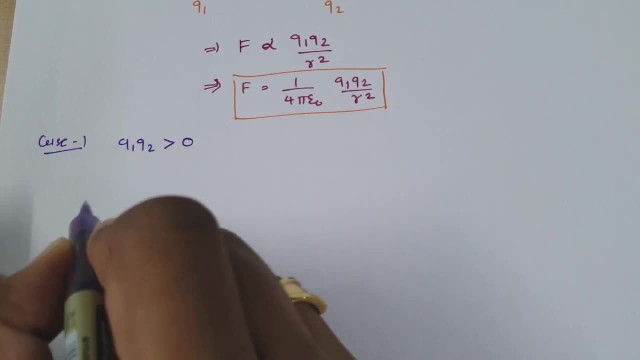 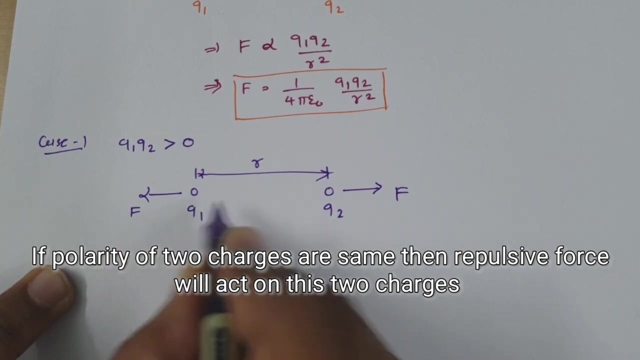 that case, even Q1, Q2 multiplication will be greater than zero. So in that case, if you observe, these are the two charges, Q1 and Q2, and distance between these two, if I say it is R, then force will be repulsive force. So you will be finding repulsive force. that will happen on 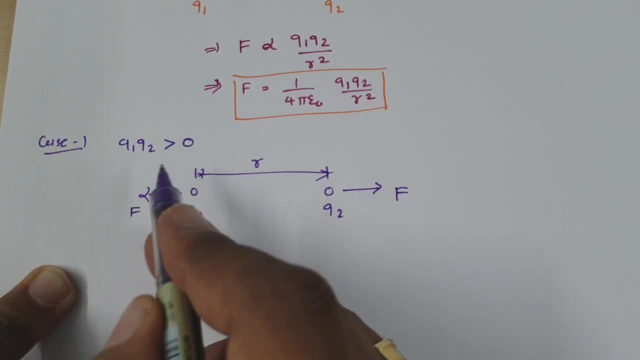 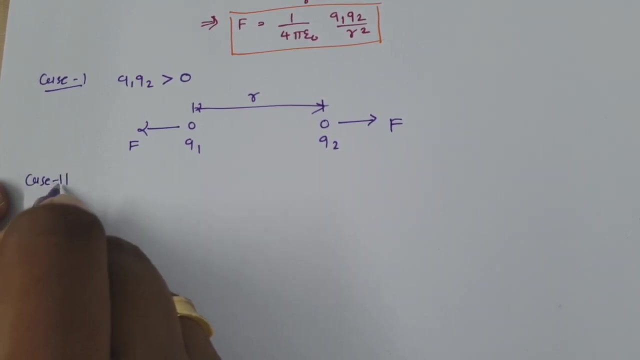 both of these charges. If polarity of both of the charges that is same, in that case there will be repulsive force that will act on these two charges. Now let us consider second case. So in second case, if I say both charges are having unlike polarity, like one charge, 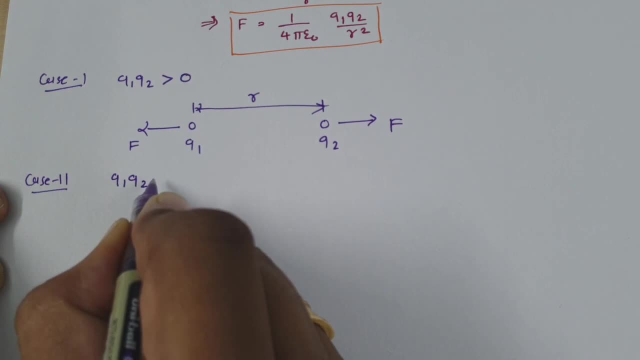 is positive and second charge is negative. So in that case Q1, Q2, that will be less than zero. So in this case there will be attractive force. So these two charges, Q1 and Q2- see both are reported by distance R, So there will be attractive force that will happen in between these two. 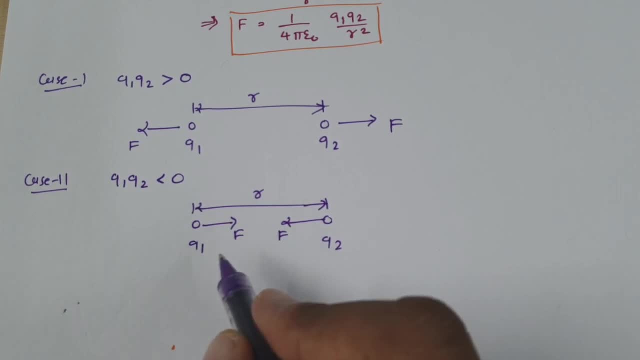 charge and force acting on both of the charges will be same and you can see the direction of force Right. So if charges are having like polarity, then there will be repulsive force, and if charges are having unlike polarity, in that case there will be attractive force, which will happen on 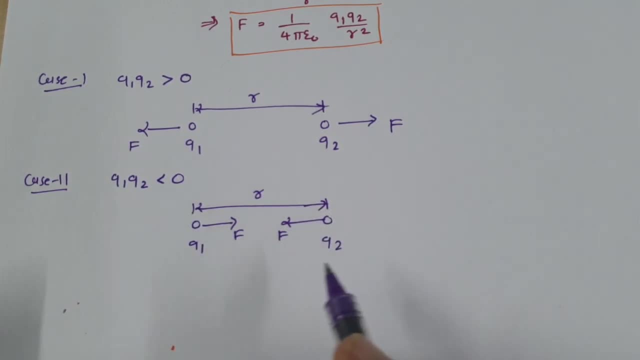 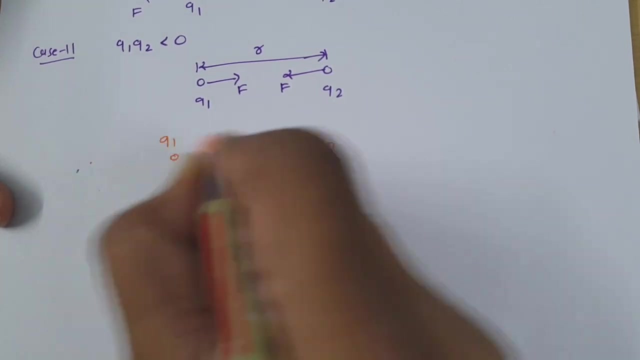 these two charges. Now let us try to understand this with respect to direction, So it will be more clear. So now I'll show you this calculation by direction. So see, if I say we have two charges, let us say this charge is Q1.. 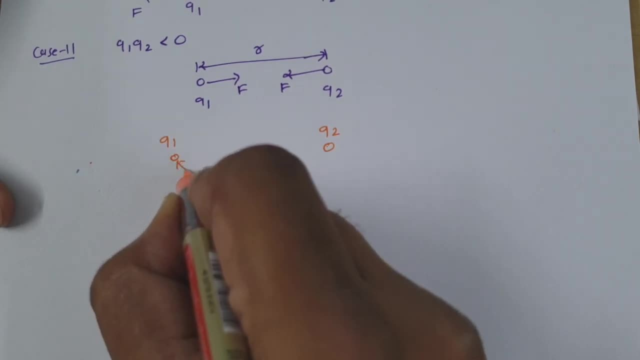 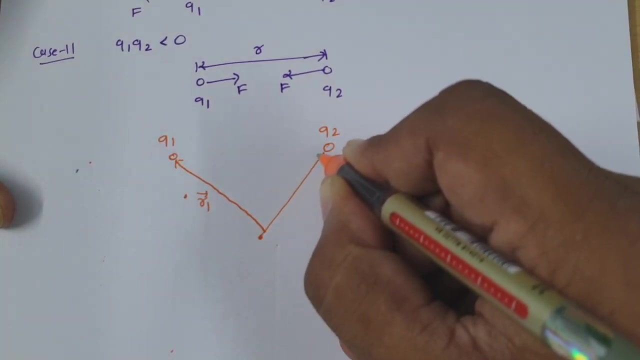 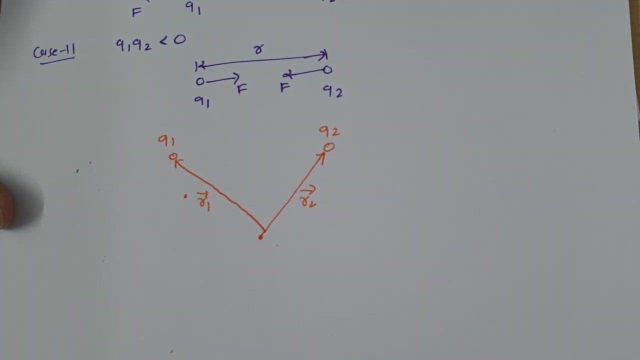 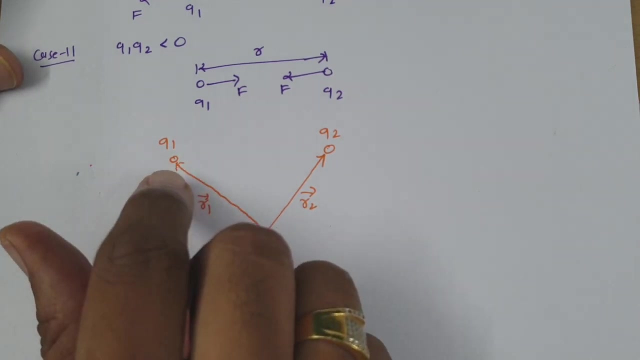 This charge is Q2 and Q1, that is indicated by position vector R1, and this charge Q2, that is indicated by position vector R2. and here, if I say Q1 and Q2, both are having same polarity. in that case there will be repulsive force. 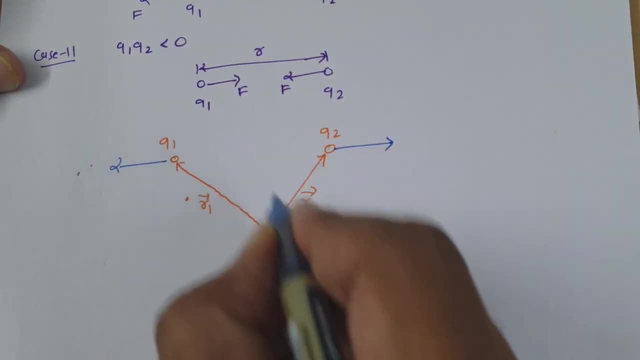 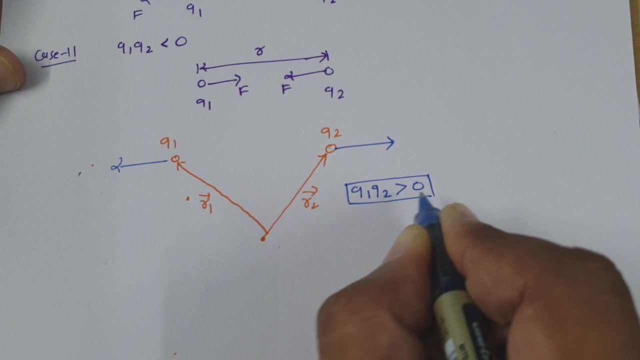 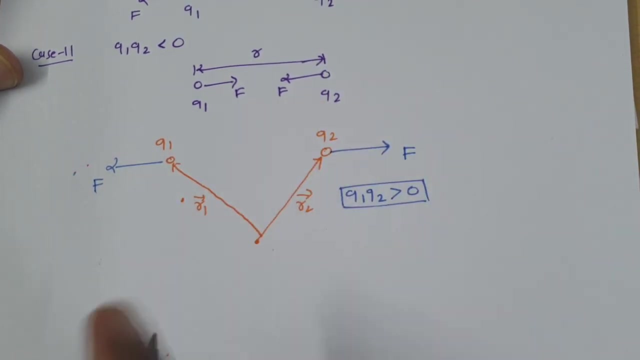 So you'll be finding- If both are here, I'm considering this case- Q1. Q2 is greater than 0. So for this case there will be repulsive force, So this force will be repulsive force. Now how to calculate this repulsive force by direction. 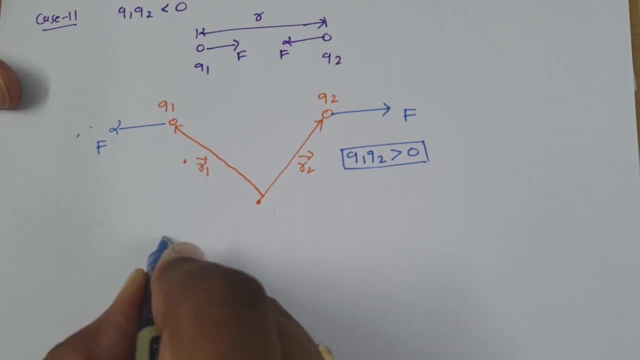 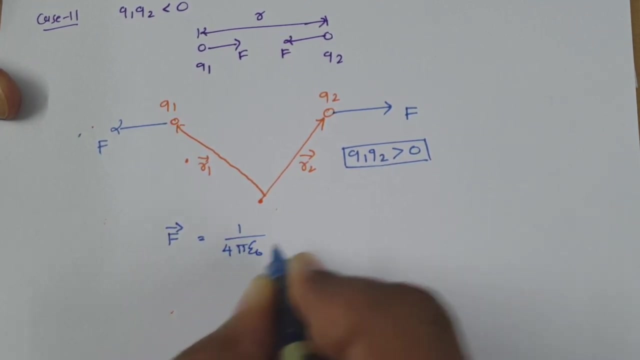 So for that see the basic formula. that is force, that is 1 by 4, pi, epsilon 0 into Q1, Q2 by R square. Now you just see, as both of these charges are having like polarity, there will be repulsive force. So on Q1, force is happening in this direction and on Q2, force is happening on this direction. 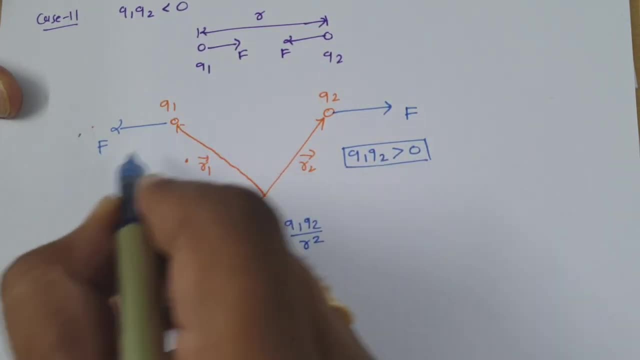 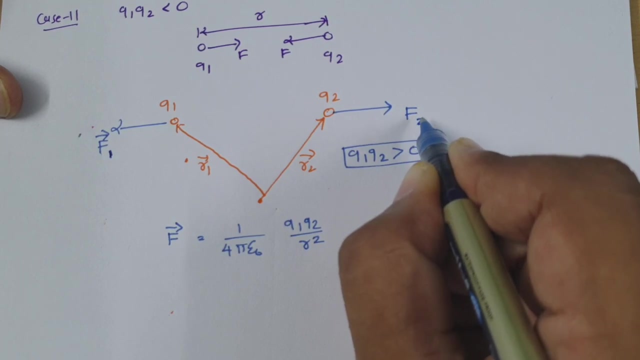 So if I say I want to calculate force acting on charge Q1, let us say that is F1 by direction and force acting on charge Q2.. Let us say that is F2 by direction. Magnitude is same but direction is opposite. So how to calculate force F1.? 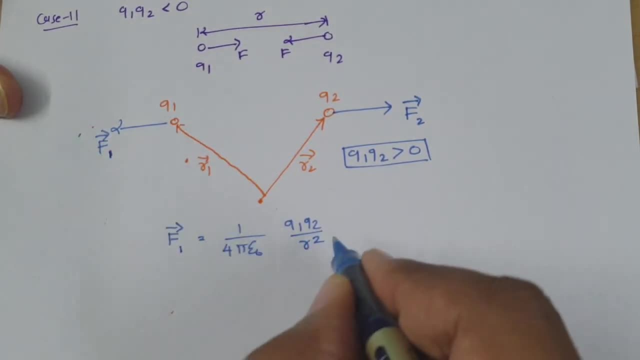 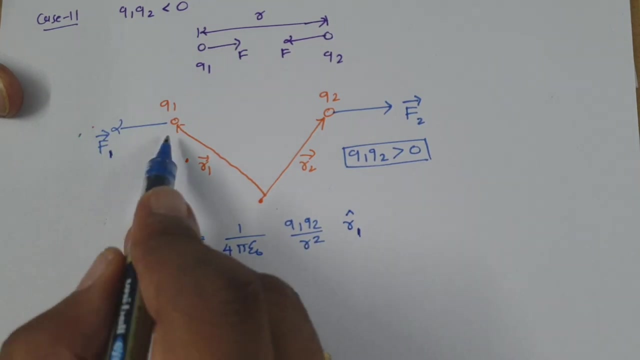 So let us say this: force F1 that is there in this direction. So we need to multiply position vector. unit position vector R1.. Unit position vector R1.. Now, what is this unit position vector R1 for a calculation of force acting on this charge. 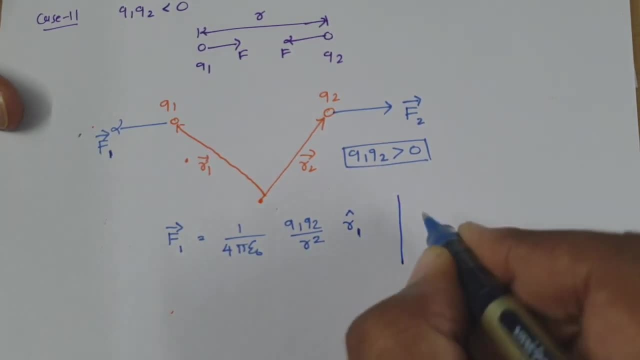 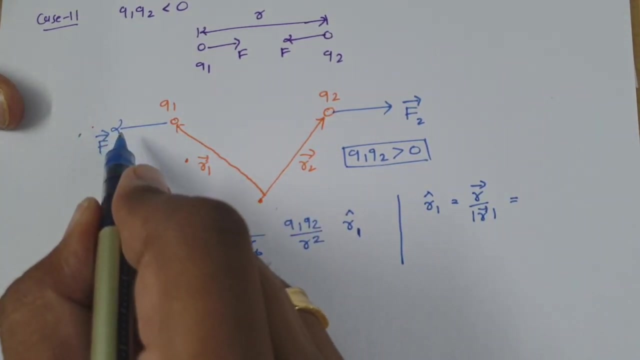 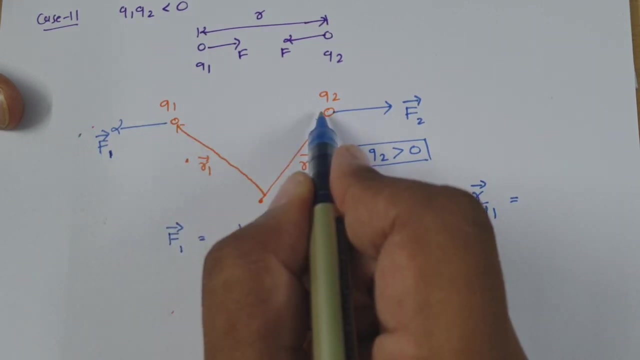 Q1.. So for that calculation, see unit position, vector R1, that is vector R divided by magnitude of vector R. So see vector R that is there in this direction. So we need to consider direction by head minus tail. So head that is Q1 and tail that is Q2.. 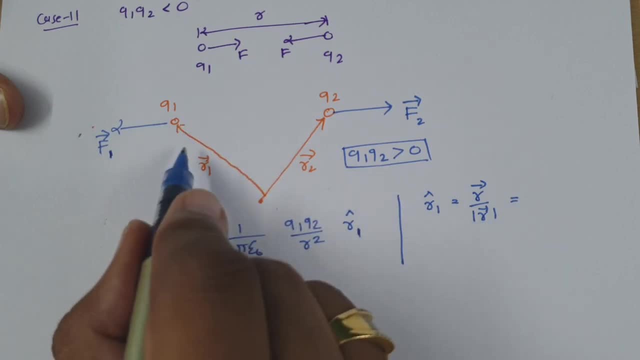 So Q1 is associated with position vector R1.. Q1 is associated with position vector R1.. So Q1 is associated with position vector R1.. And Q2, that is associated with position vector R2.. So direction on force acting on this, that is R1 minus R2.. 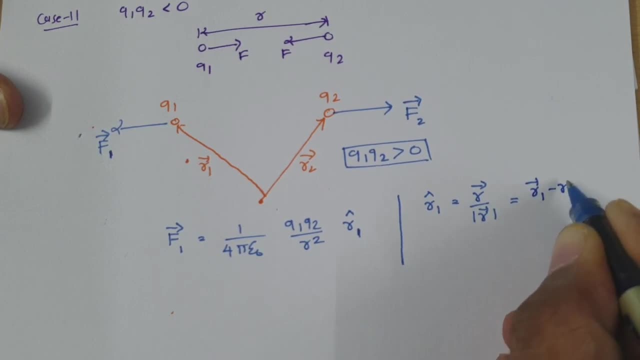 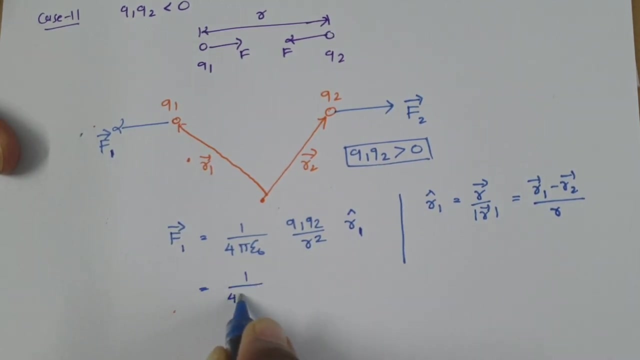 So here you need to consider this direction: R1 minus R2, and divide by magnitude, that is R only. So see now, if you place this formula over here, So now this formula will get to 1 by 4 pi, epsilon 0. So this is R1 minus R2.. 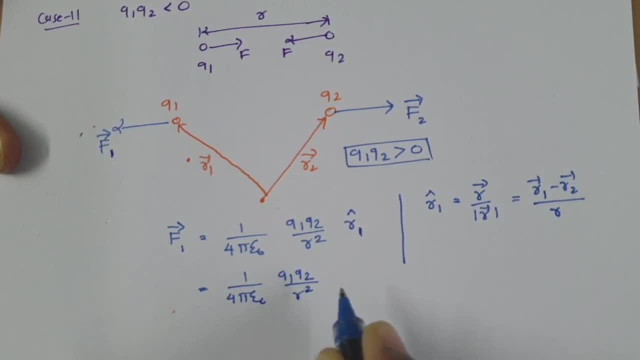 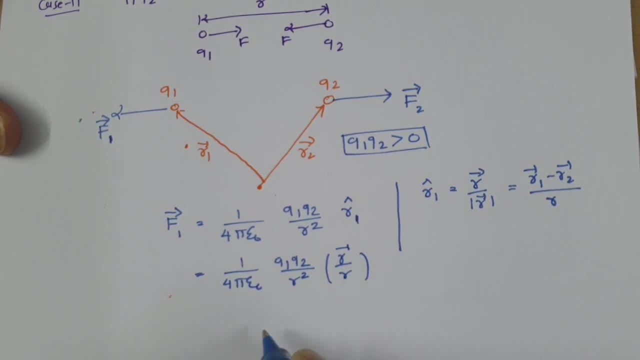 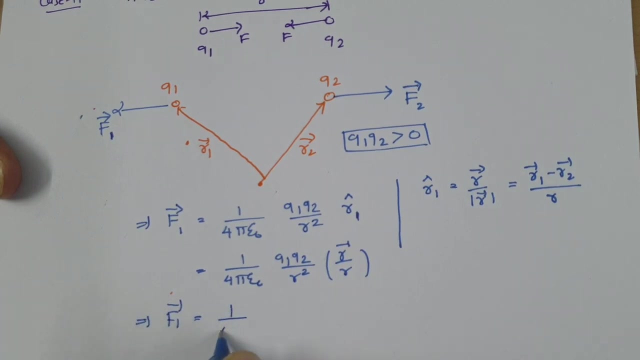 Q1, Q2 by R square into vector R divided by magnitude, vector R. So now by direction, this force, now that will change to 1 by 4 pi, epsilon 0.. Q1, Q2 by R: cube into vector R Where vector R is R1 minus R2.. 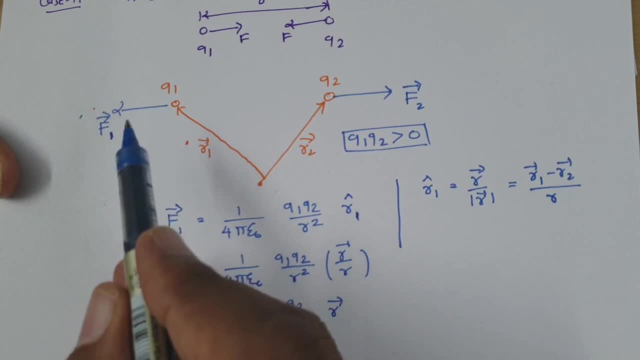 In case of you calculate 4 pi, epsilon 0.. force acting on charge q1 and similarly we can have a calculation of direction for force acting on charge q2, and that will be if I say that magnitude will be same, but you will be finding. 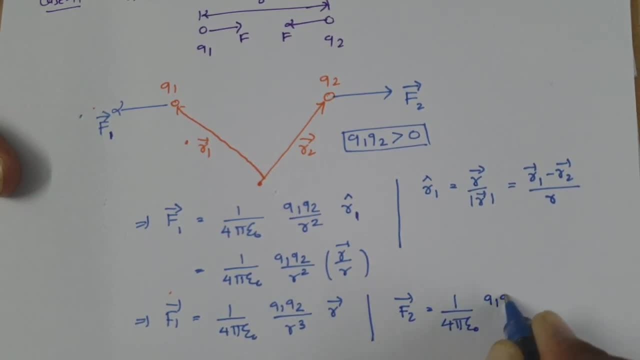 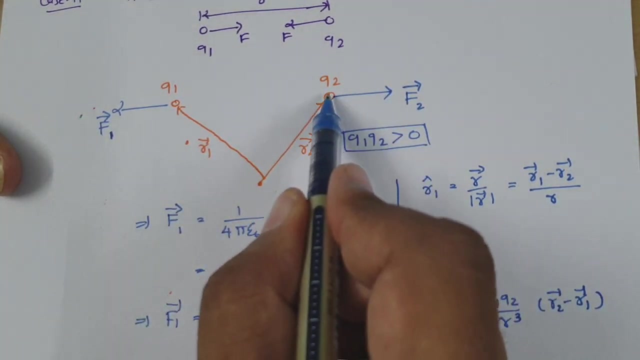 that direction is opposite. so 1 by 4 epsilon, 0, q1, q2 by r cube, but now you will be finding direction- is vector r will be now vector r2 minus vector r1, and that is happening as per head minus tail, where head is actually, this means r2 minus r1. see, that is how it is happening. 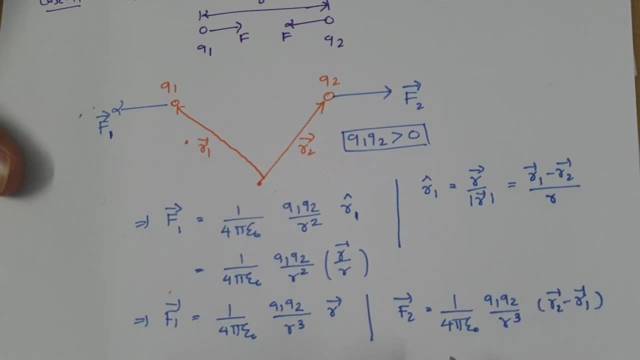 now why I am explaining this. the reason is I have seen students were asking one question, always like see. in books sometimes that is written as per formula: 1 by 4 epsilon 0 into q1, q2 by r, cube into vector r2.. See actual force is q1, q2 by r2. sometimes in books you will be finding 1 by 4 epsilon 0. 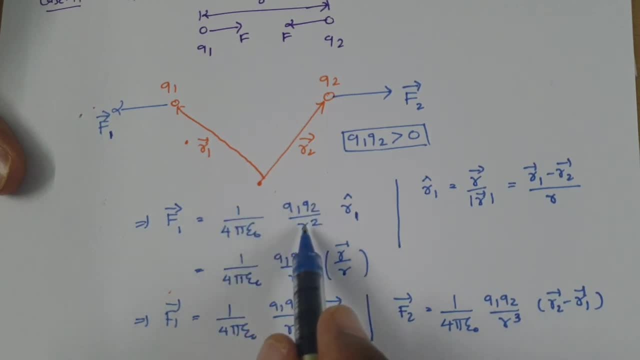 that is written as k, so k q1, q2 by r2 and in some formulas you will be finding it is k q1, q2 by r. cube into vector r. so that is happening as per unit vector. why? the reason is: see this is direction. 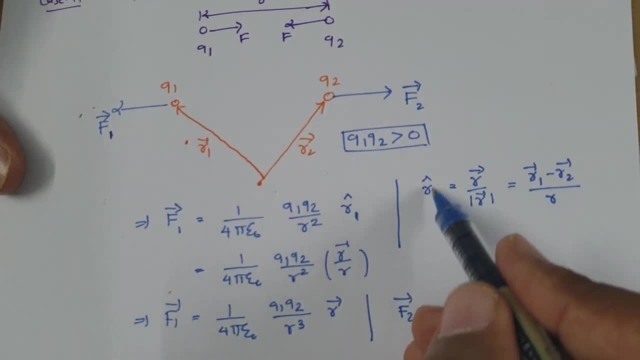 vector. this is direction vector, so direction vector is direction vector, So that will get to unit vector. that's why this formula is getting changed by 1 divided by r cube instead of r square. so this is what you need to keep in your mind. sometimes you 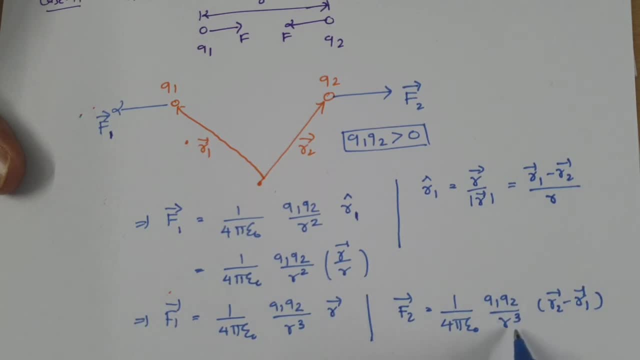 will be finding it is written as per 1 by r cube, right, but that r cube is happening because of unit vector. so this is what we need to consider when we calculate examples. now let us try to solve one problem, so it will be more clear. 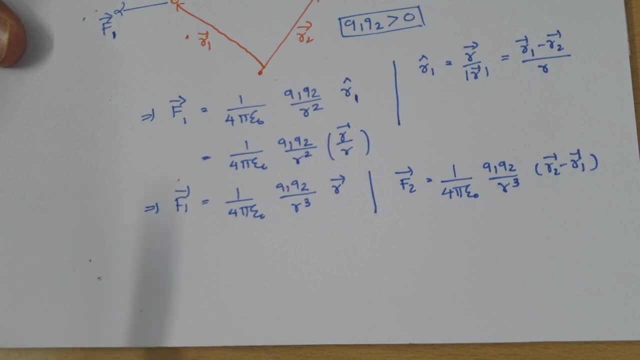 So let us try to solve one problem, so it will be more clear. So here we have been given with one question, and that question is: we have two charges. one charge is q1, and that is 1 microcoulomb, and second charge is q2, that is 2 microcoulomb. 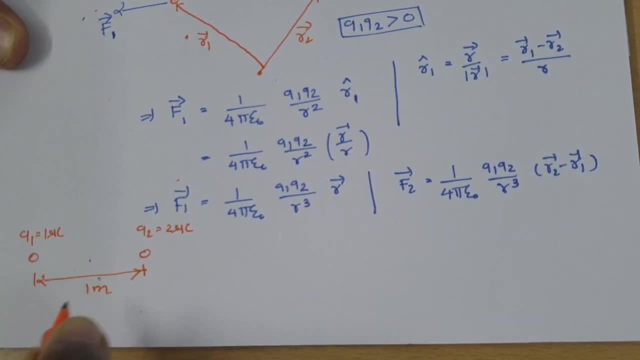 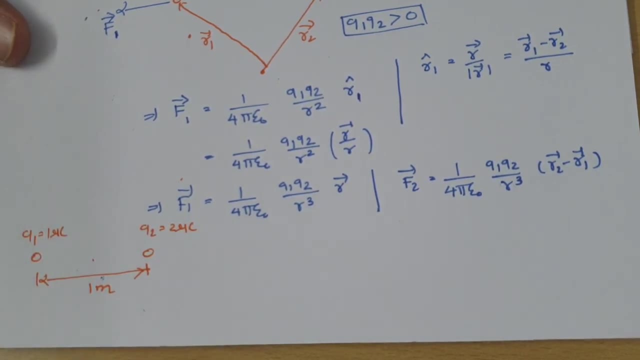 and both are aparted by distance 1 meter. So what is the force which is acting on q1? so first of all, we need to understand one thing: See Here This q1 and q2, both are having same polarity. so as both are having same polarity, this force. 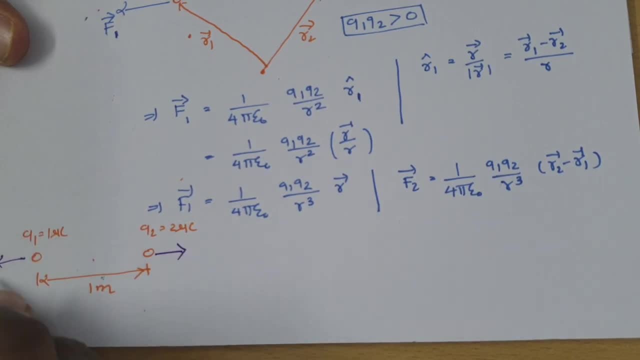 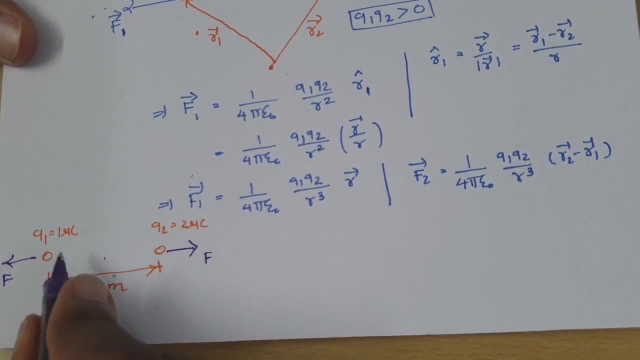 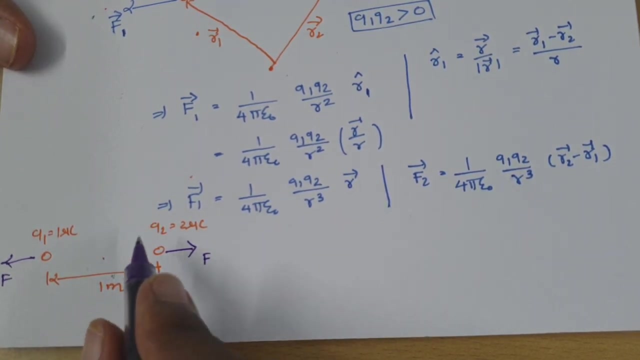 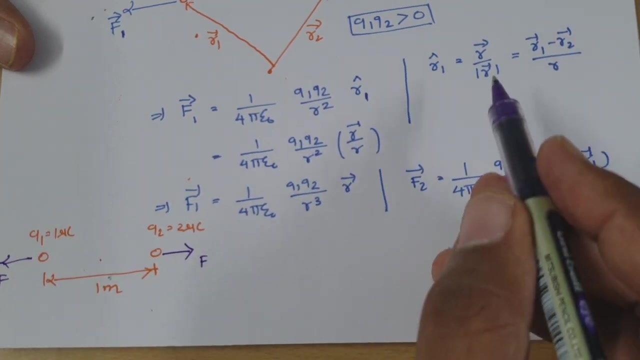 will be repulsive force. So on q1 as well as q2 force will be repulsive force, as polarity of both charges are same and here position vector is not given, so as if position vector is not given, we can only calculate magnitude If position vector is being given. in that case you can find position vector as per I. 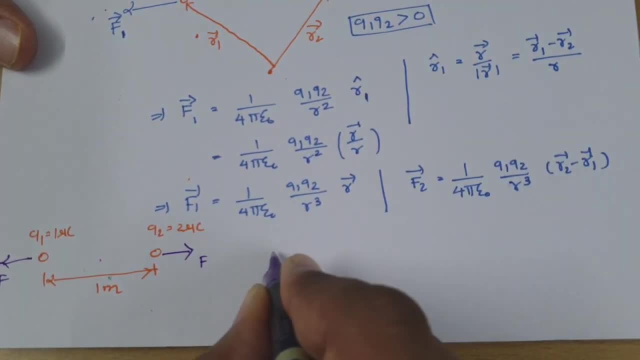 have explained here. So this force calculation, that will be F, is equals to 1 by 4 pi epsilon 0, q1, q2 by R square. this is a magnitude, and this will be 1 by 4 pi epsilon 0. all together, that is 9 into. 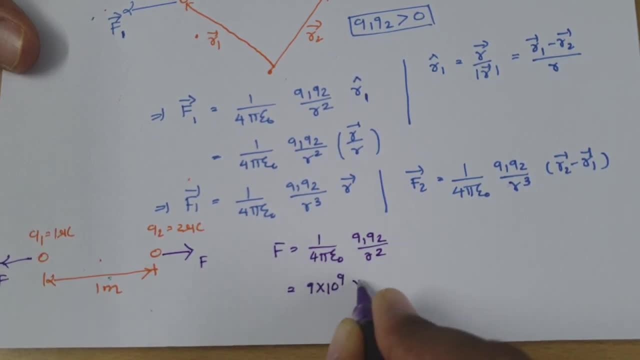 10 to the power 9 in SI, and q1, that is 1 microcoulomb, so 10 to the power minus 10 to the power minus 9.. Q2, that is 2 microcoulomb, so 2 into 10 to the power minus 6, divided by R square, R square. 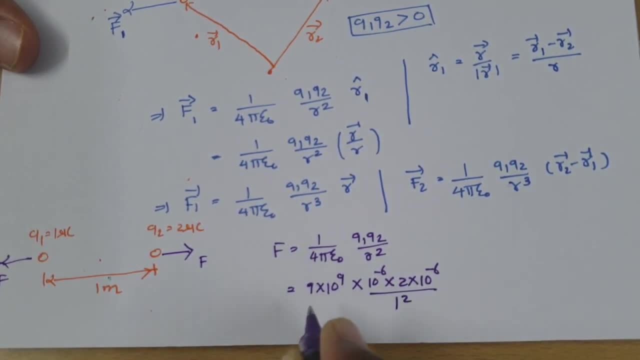 is 1 meter, so I am writing 1 square. So if you calculate this, 9 into 2, that is 18 into 10 to the power 9 and 10 to the power minus 6 minus 6. so 9 minus 6 minus 6, that will be 10 to the power minus 3..